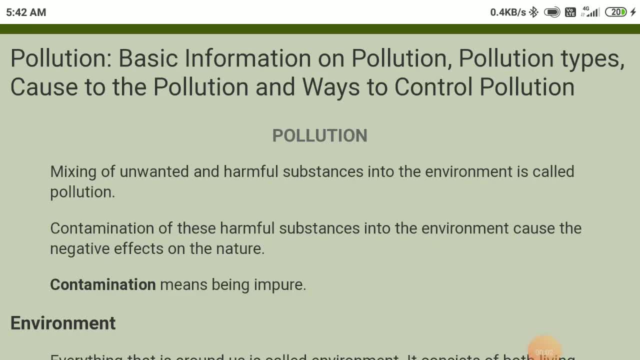 Hello everyone, Welcome to the top lessons. Today's topic is pollution. Today we are going to talk about basic information on pollution, types of pollution and causes to the pollution and various ways to control it. So what is pollution? Pollution is mixing of unwanted 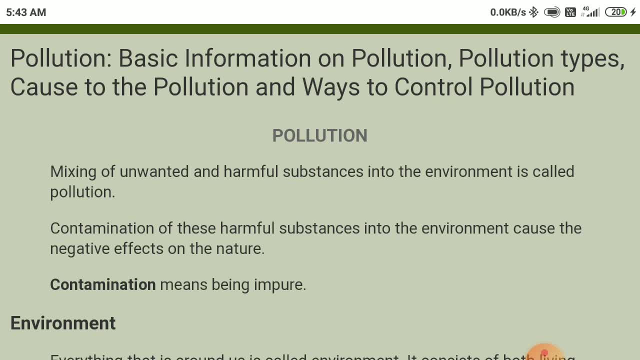 and harmful substances into the environment, or anything which is already present in the environment, but the amount or quantity of that particular substance is more than required, that is also considered as pollution. So contamination of these harmful substances into environment causes the negative effect on the nature. Contamination means being impure. 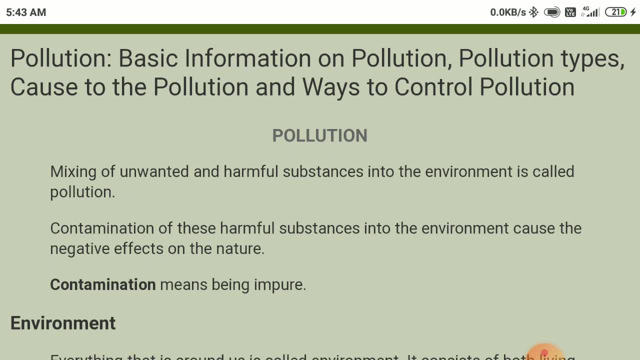 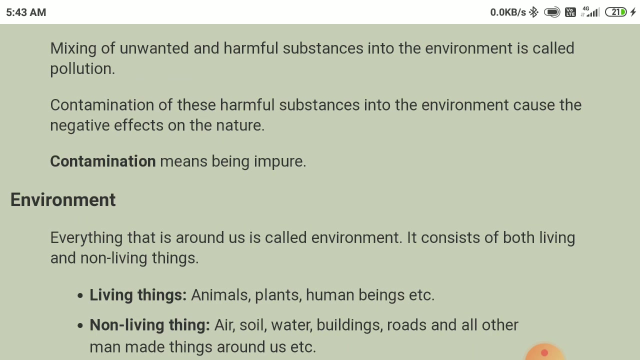 or getting mixed with the impurity. So in environment, whatever harmful substances are present in the environment, they are considered as pollution. So pollution is getting mixed. They are putting negative impact. For example, climate is changing, natural calamities are also coming, So that is how this impact of pollution is very high on the nature. So 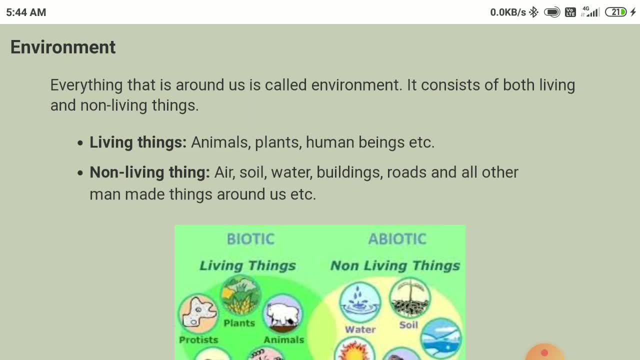 let us talk about environment. Environment is anything which is around us, Anything. it can be living things, non-living things. Living things are called biotic elements of the environment, Non-living things are called abiotic elements. So living things can be like animals, plants. 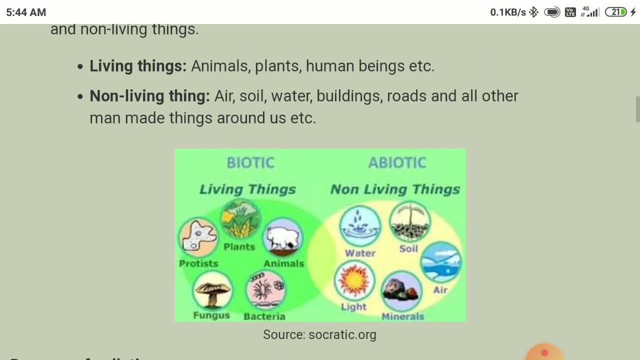 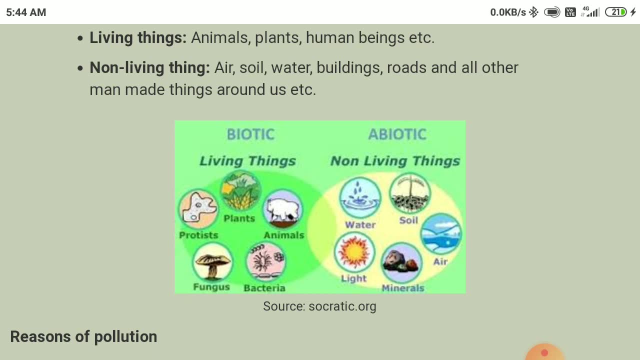 human beings. Few examples more are given in this picture, like protists, bacteria, fungus. So these are microorganisms. These are also part of biotic elements of the environment. So in non-living things or abiotic things we have water, soil, air, minerals, light. 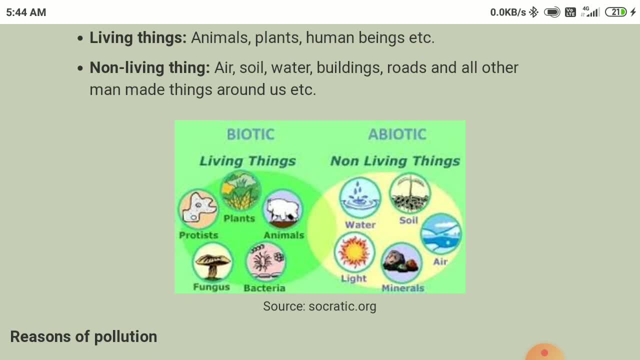 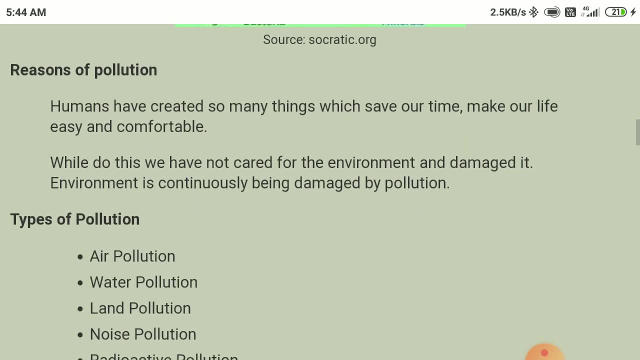 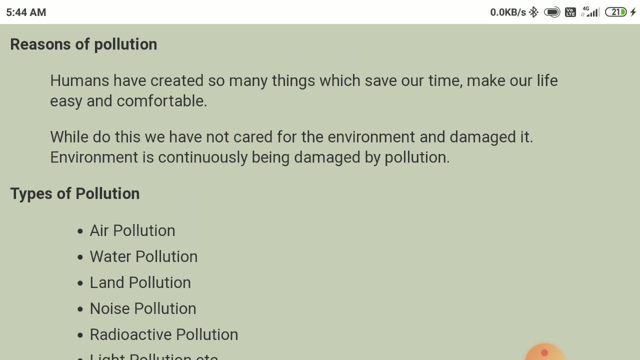 buildings, roads, anything which does not have any life, So these can be included in the non-living or abiotic elements of the environment. So, because of the pollution, this environment is getting contaminated and it is having severe effect on it. So let us talk about reasons of pollution In general. we are talking about 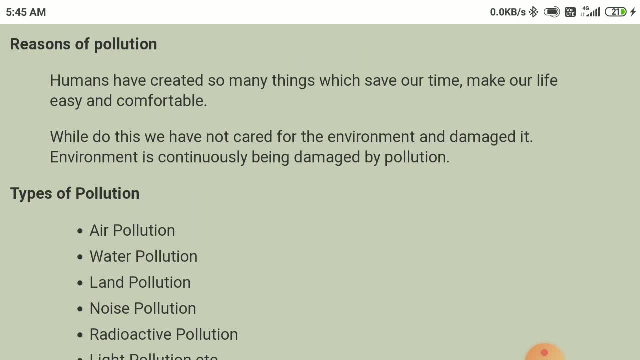 one reason, that is for our convenience. humans have created many things like vehicles, vehicles, vehicles. So we are making vehicles to make our life easy and convenient, but in doing so we are using fuel in our vehicles which is releasing gases into the atmosphere, which is causing the air pollution. Similarly, we are doing so many other things, like in the 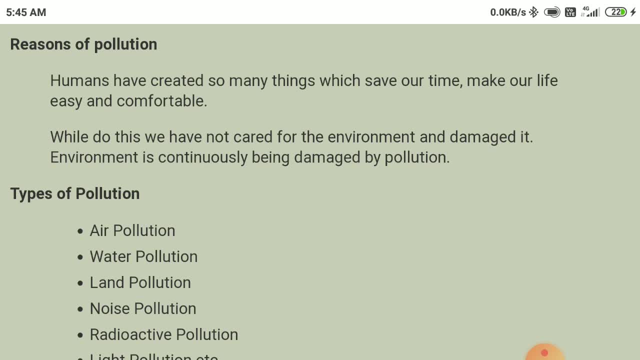 factories or in the industries we are using various chemicals. These chemicals are getting released into water. That is causing water pollution. These factories are also making noise- various types of noises, which are not good for the nearby environment. That is how we can say it is creating noise. 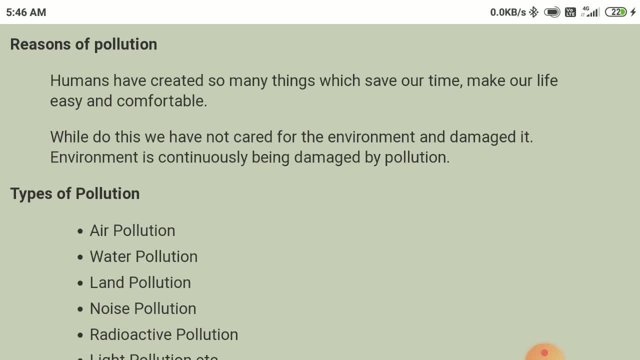 pollution. Similarly, the vehicles are also creating noise pollution. Jet planes, if you have seen any that also cause too much of noise pollution And land pollution. In doing that, we are also using pesticides, fertilizers in excessive quantity to increase our productivity in agricultural fields, But those are having negative impact and they are getting mixed. 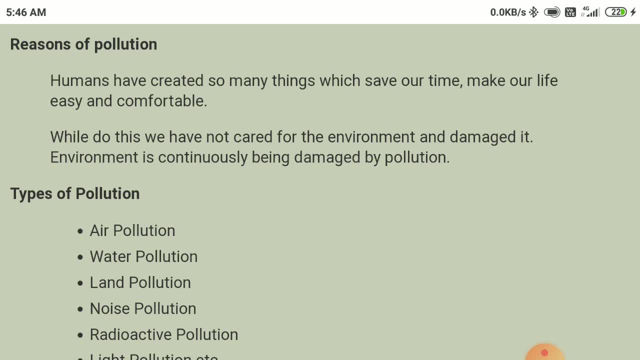 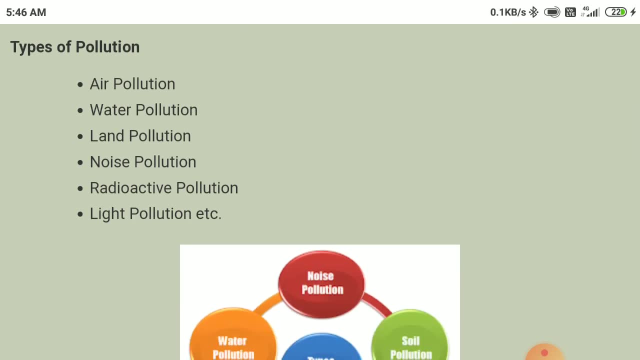 into the land and causing negative impact. Okay, similarly, we are going to talk about the types now. So we have air pollution, water pollution, land pollution, noise pollution, radioactive pollution, well as light pollution. so these are some important types of pollution. so 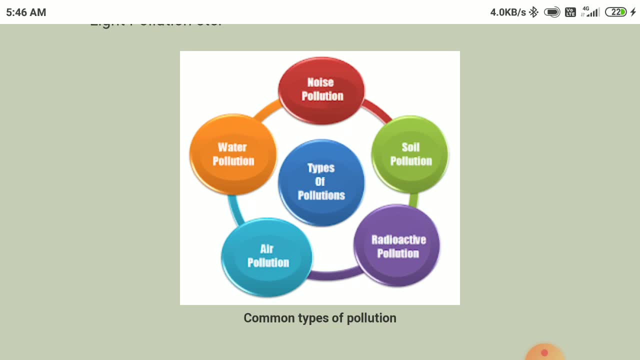 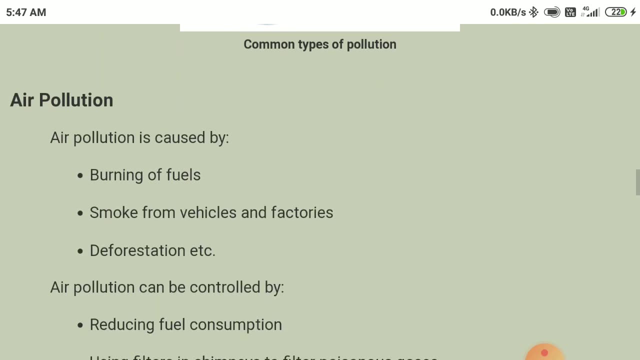 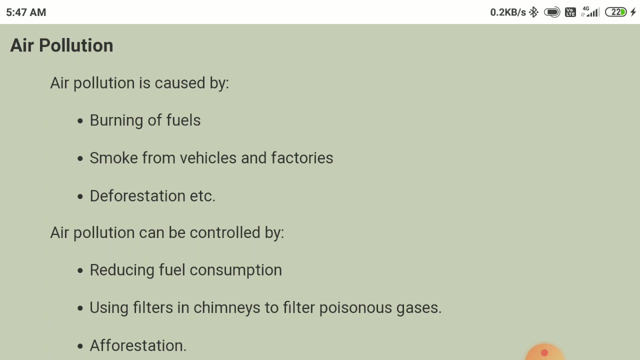 this picture also shows the common types of pollution which are frequently used in the discussions. okay, so let us talk about air pollution. we are going to talk about few causes and few ways to control it. the main causes and ways to control it. let us talk about the causes first. so main cause of air pollution is burning. 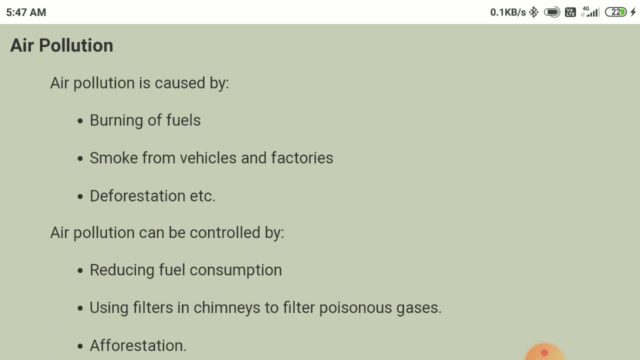 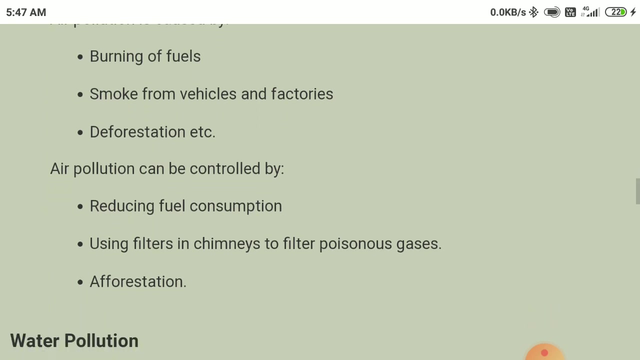 of fuels in vehicles or at home, also, like a coal or anything which we are burning to get the energy or smoke from the vehicles, factories, deforestation. deforestation is one of the, you know, biggest cause for air pollution. so these are the causes now, if we talk about the ways to control it, so reducing 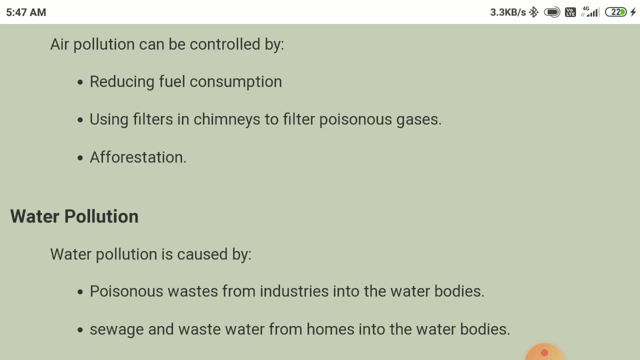 the fuel consumption, using the filters in chimneys to filter the poisonous gases coming out of the chimney. in that way, we can actually, you know, filter out the harmful- you know harmful- elements, or the small particles which are present in the smoke coming out of the chimneys, because those small particles that are 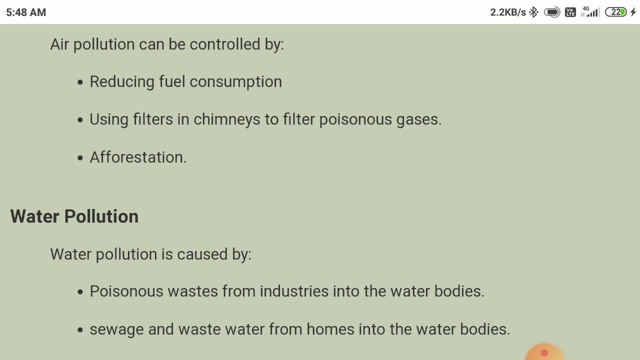 if they get mixed into the environment, those are not actually visible, but they gets deposited on the layers of leaves- if you have seen somewhere- and that actually we, we breathe in those particles into our lungs, so that creates various problems okay, like asthma. so these are the reasons. that's why we can. 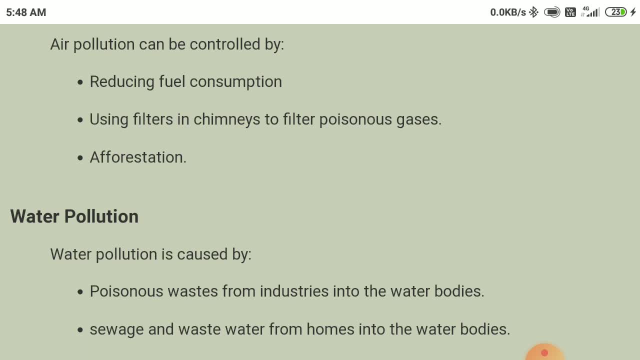 use the filters in the chimneys to filter out the poisonous gases also. and afforestation? afforestation is like the opposite of deforestation, so we have to plant as many as possible and the trees as many as possible so that plants actually take, take in the carbon dioxide and release oxygen so that we 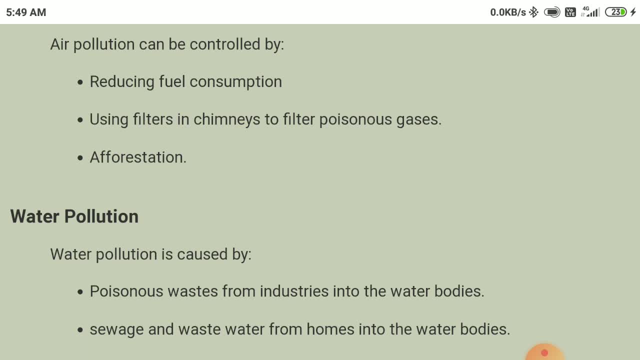 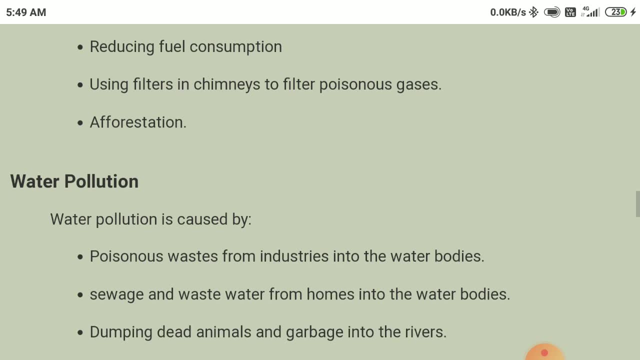 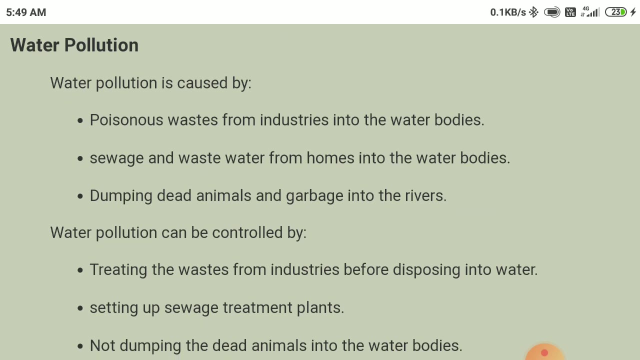 can reduce the quantity of co2 in the atmosphere, or carbon dioxide is the atmosphere, and increase the availability of oxygen. next type of pollution we are going to talk about is water pollution. water pollution is caused by poisonous waste materials that are released from industries and that are directly disposed into water bodies. water bodies like 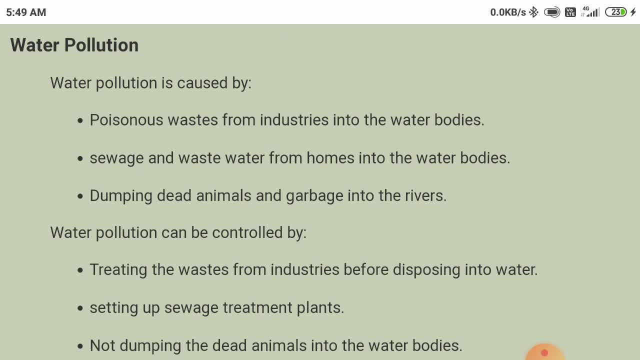 rivers, lakes, ponds, seas, oceans- okay, so sewage and waste water also from they are coming from homes and from, you know, various buildings or industries also. so these sewage water and waste water you know cause the pollution in what water water and dumping dead animals, garbage into the rivers. 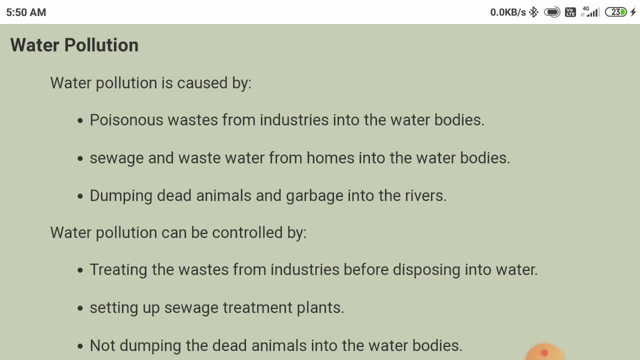 this is. this has been very serious issue because, like many people throw uh dead, you know, dead bodies of animals or garbage into rivers very frequently. that is why in india, we have all the rivers getting polluted up to a very high level. ganga is one example. river ganga is one example. 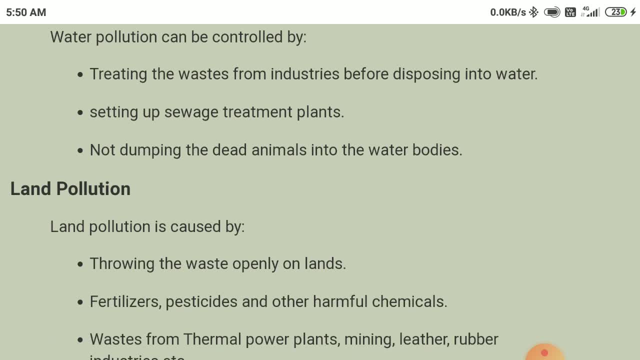 so there are ways to control the water pollution, which is treating the waste which is coming out of industries before depositing, depositing, disposing into water and setting up sewage treatment plants so that we do not directly put this sewage waste or sewage water into the rivers or the water bodies and not dumping the dead animals into the water. 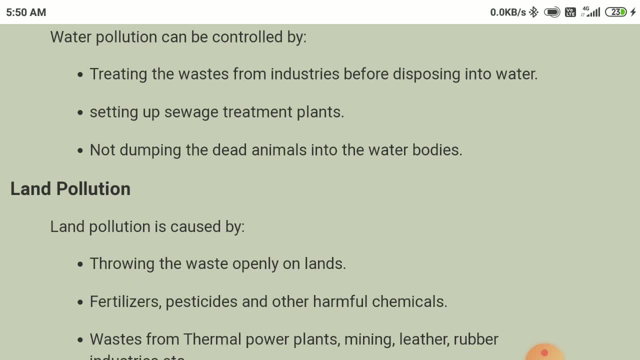 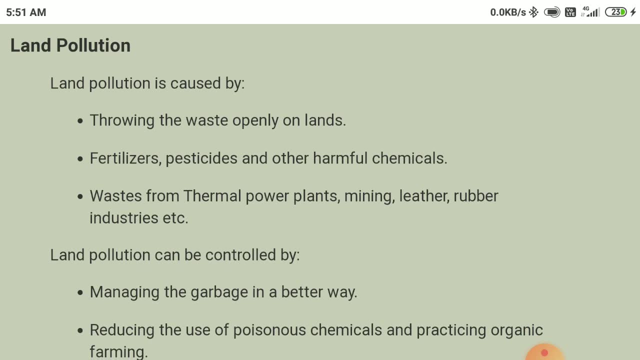 bodies. so, whatever are the causes, we just have to negate that, and that is how we can control the pollution. next thing is laxative pollution, and that is how we can control the pollution. next thing is land pollution. land pollution is caused by throwing waste openly in land. so 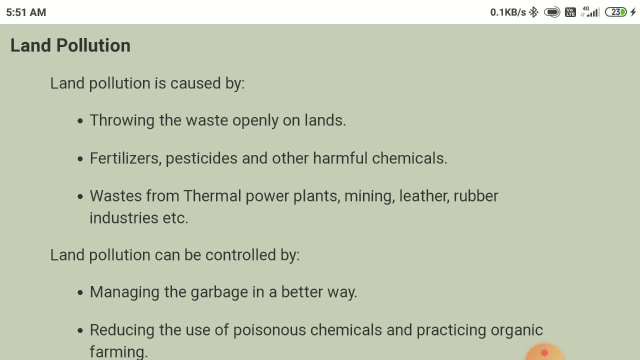 whatever the waste material we are generating out of our households, factories or industries, that is actually directly thrown on the open areas, so that get that creates the pollution on land. similarly, we are using fertilizers, pesticides and other harmful chemicals in our agricultural activities in the fields. that is, get that is mixed with the land and with the soil that creates. 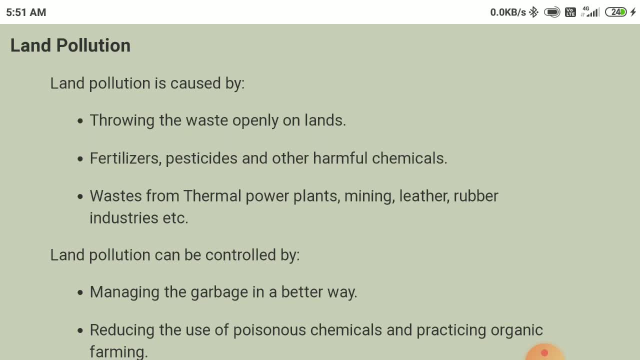 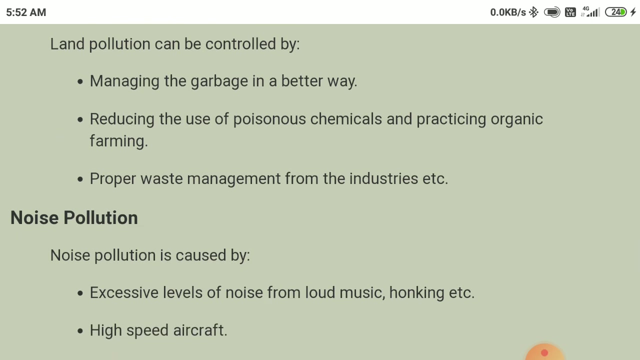 negative effect. and we also have waste materials coming out of the thermal power plants, like the ash from the burnt coal and from mining, from leather and rubber industries that also. so these are the harmful elements getting mixed with the land and making land, you know, polluted or not useful for any use. so land pollution can be controlled. 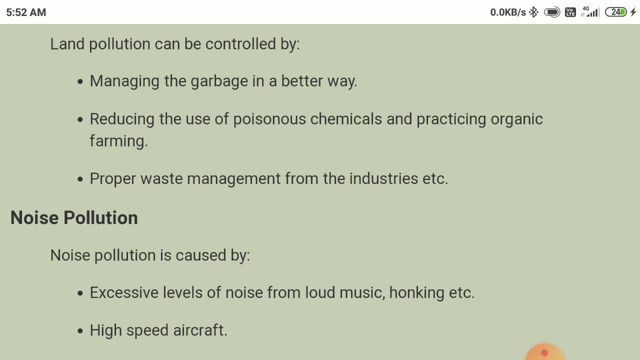 by managing the garbage in a better way. whatever the garbage we are generating, we have to manage it a proper, in a proper way. proper disposal places should be created for that. we should not throw the garbage anywhere. everywhere we should have some specific place and that should also be properly managed now. 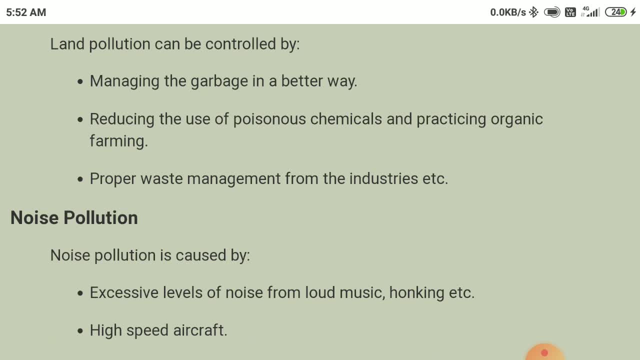 the land pollution is by reducing the use of poisonous chemicals and practicing organic farming. so organic farming these days is very famous phenomena which is happening because of the various type of disease you know happening because of this poisonous chemicals being used in agricultural. so people are moving towards organic farming. that is very useful for us where. 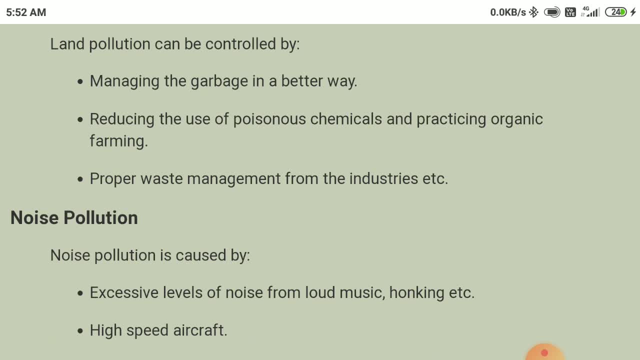 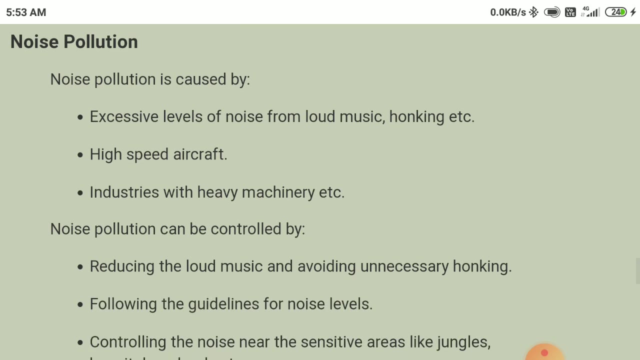 we are not using any harmful pesticides or fertilizers. next thing we can do is to control land pollution, is proper waste management, as I told. so these are the ways to control the land pollution. next type of pollution is noise pollution. so noise pollution is caused by excessive levels. 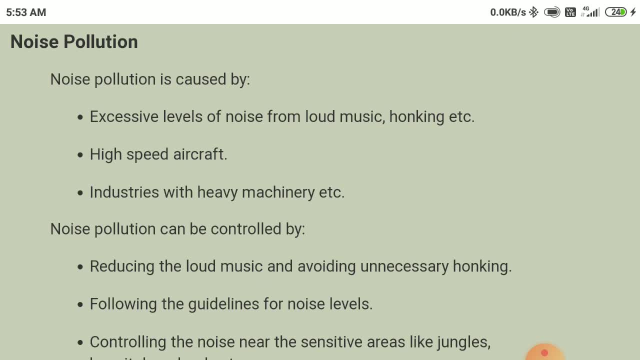 of noise from loud music, honking in the traffic. unnecessarily. we do that, that we blow horns, even if we are knowing that there is a jam in the traffic, but it's still. we keep on blowing the horns or keep on honking. another cause can be high-speed aircrafts, which creates so much noise. industries with heavy 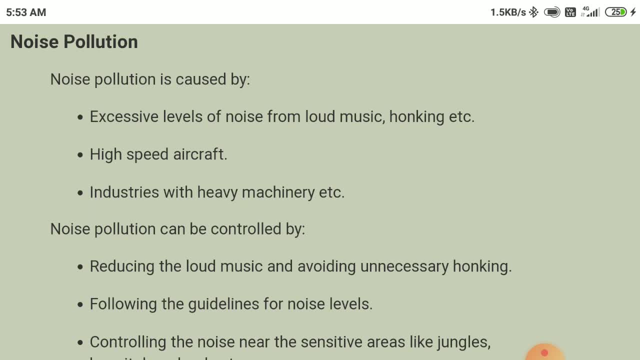 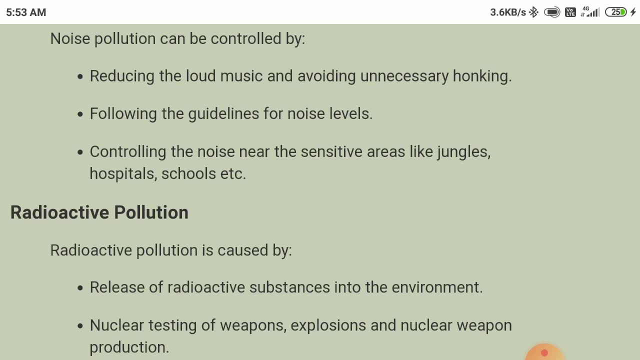 machineries also create so much noise. so these are the main causes which creates noise pollution. now, noise pollution can be controlled by reducing the loud music and avoiding unnecessary honking in the traffic, following the guidelines for noise levels we should- we should- be making noise up to a certain level, not beyond that, because after that it creates. 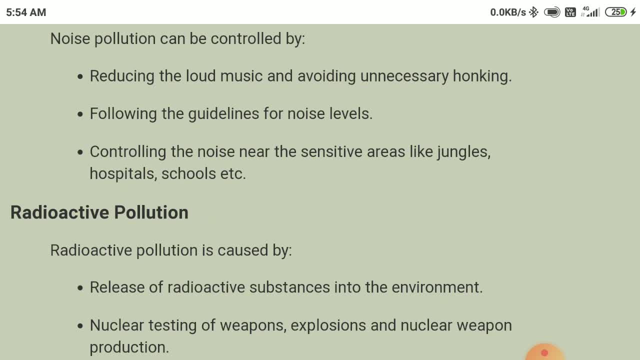 negative impacts. controlling the noise near the sensitive areas like jungles, because animals are there, they get afraid of it and they, you know, have negative effect on them. hospitals, schools, hospitals are another impôrde spamming software to reduce the noise in cities or cities, other places of the world, so we can catch the noise of the wild burn, since the animals complain. it is dangerous to the environment and 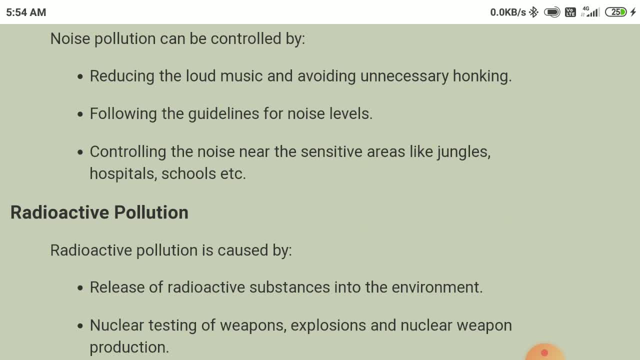 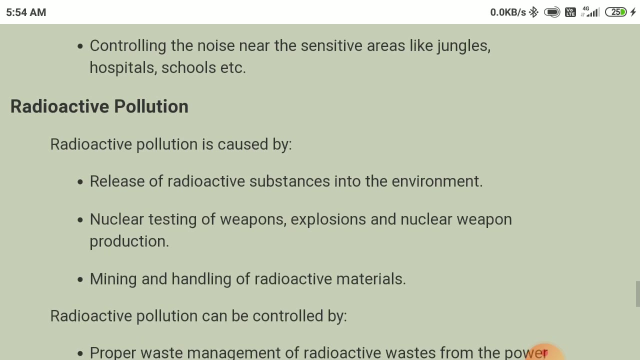 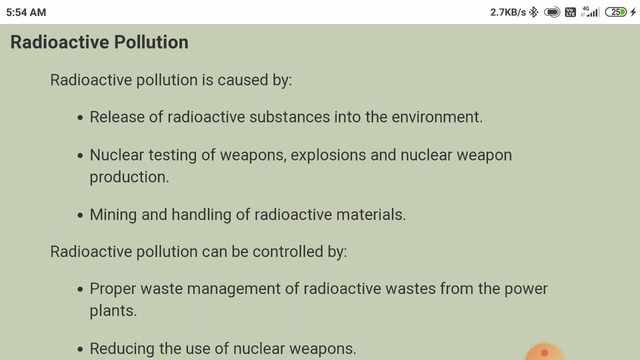 sensitive places, like same as schools. so these are the you know areas. at least here, near to those areas, we should not have any noise, noise pollution, because there it causes more effect. next type of pollution is radioactive pollution. that is mainly caused by a radio release of radioactive substances into the environment, nuclear testing of weapons explosions, nuclear 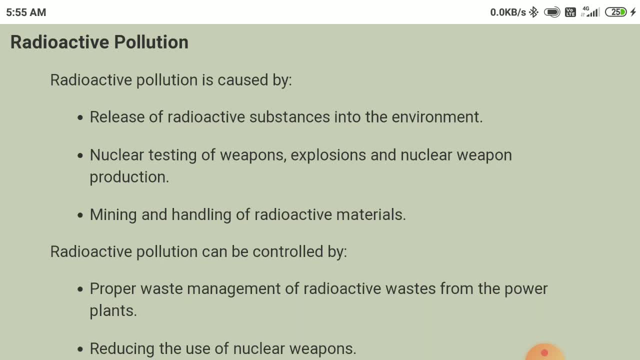 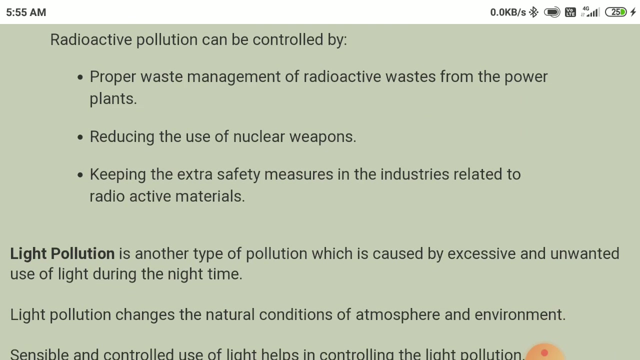 web, weapon productions, mining and handling of radioactive material. so basically wherever we are dealing with the radioactive materials which release the radiation into the environment, because of that radiation, the pollution, radioactive pollution is caused. so we can control radioactive pollution by proper waste management of radioactive waste from power plants, from nuclear power plants, whatever. 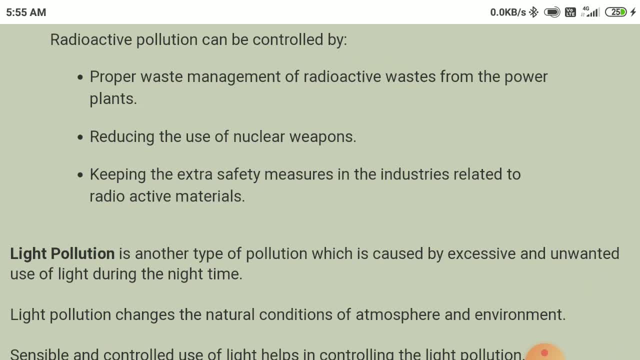 radioactive waste is being generated. that should be properly managed because that is very harmful. next thing we can do is to reduce the use of neck nuclear weapons, but it is difficult because every country is, like now, planning to have nuclear weapons and whenever I use them, whenever required. but we have to find a way where we can. we do not use the nuclear weapons and nuclear weapons use of nuclear weapons are reduced. uses of nuclear weapons are reduced. another thing we can do is to keeping the extra safety measures in the industries related to radioactive materials. so whenever we are dealing with radioactive materials, we have to keep extra measures so that it does not cause any harm to the environment. 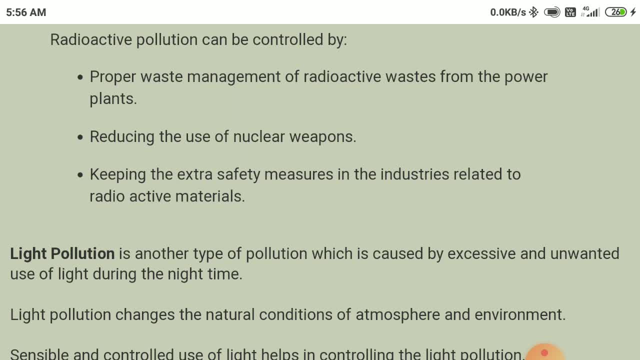 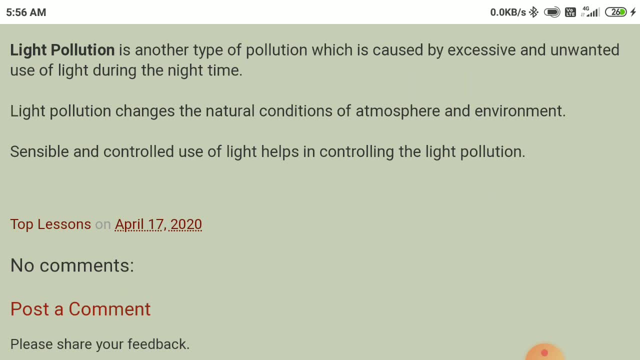 the environment in the emergency time. now. light pollution is also another type of pollution which is caused by excessive and unwanted use of light during the night time. you might have seen in functions or you know other places. wherever they are unnecessarily extra light is being used just to make. 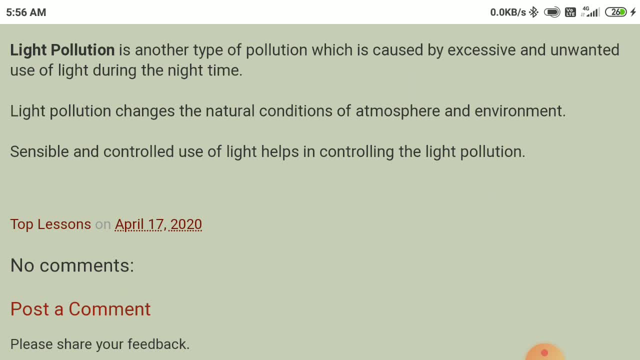 the place bright, but sometimes it is used overly. so overuse of light is also not good for our environment, because during the night time, when this excessive and unwanted light is used, the one thing you observe is that we are not able to see in the sky. another thing: because of this light, because light also